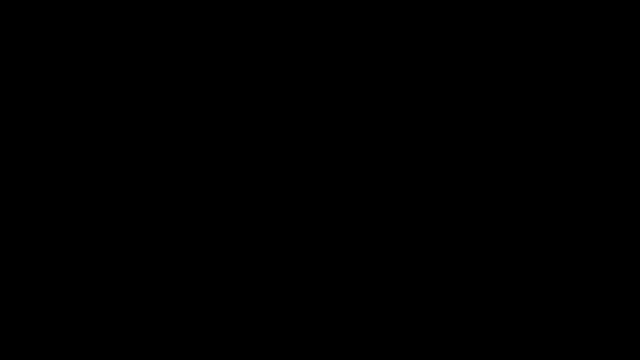 In this video we're going to talk about how to determine if a series will converge or diverge. So here's an example. Let's say, if we have the infinite series of 2n, Will this series converge or diverge? What would you say Now, before we? 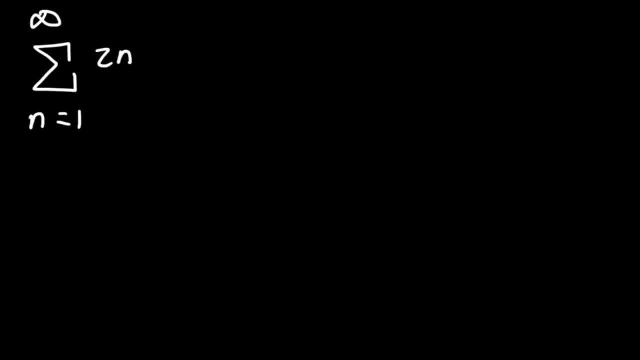 get into it. you need to know the difference between a sequence and a series. So in this example, the sequence, a sub n is 2n. So if you list out the terms of the sequence, the first term, a sub 1, is going to be 2, the second term, 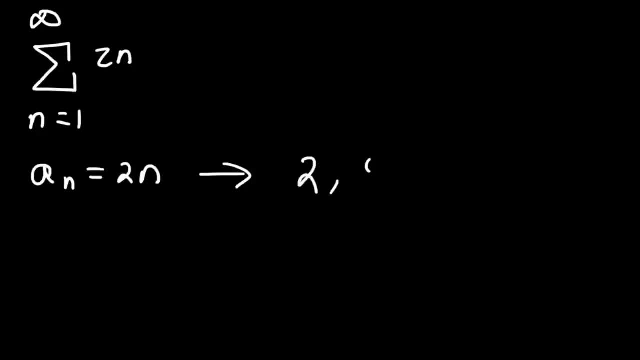 a sub 2 is going to be 2 times 2, which is 4,. the third is going to be 2 times 3, which is 6, and then 8, and so forth. And so here we have a sequence of terms Now. 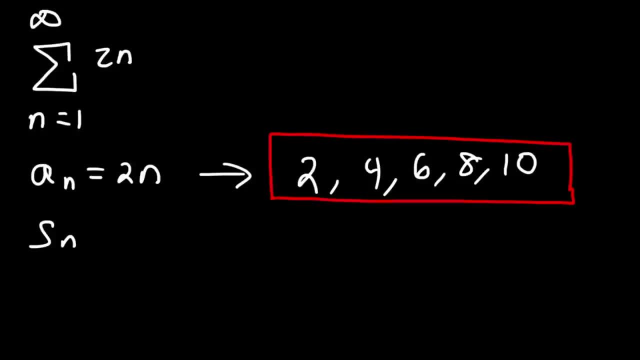 s sub n relates to the partial series of a series. So if you list out the terms of a series you're going to get a partial sum. So for example, s sub 1 is just a1, which is 2.. s sub 2 is the partial sum of the first two terms, So that's a sub 1. 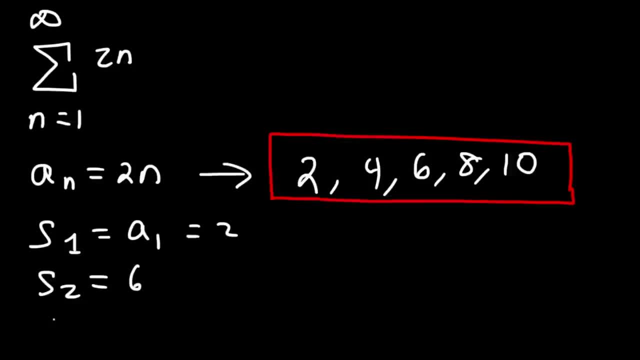 plus a sub 2, which is equal to 6.. s sub 3 is the sum of the first three terms, which is 12,, and s sub 4 is the sum of the first four terms, which is going to be 12 plus 8 or 20.. 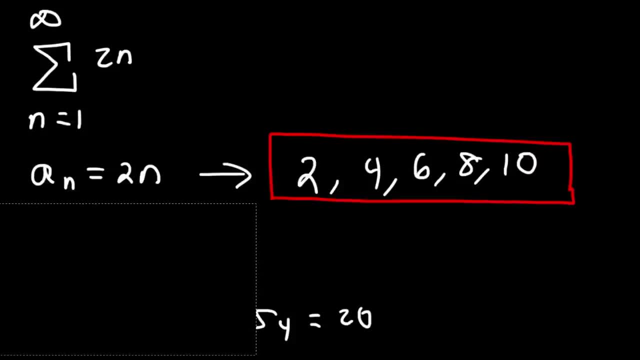 So, if we want to, we can write out a sequence of partial sums, So s sub n. we can say s sub 1 is 2, s sub 2 is 6, s sub 3 is 12,, s sub 4 is 20, and if the 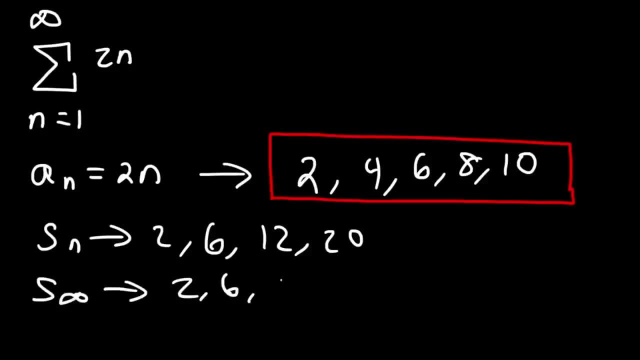 sequence goes into infinity. this will keep on going forever, And so this is termed an infinite series. So this is equal to s sub infinity. It's the sum of the first infinite terms. Now how can we tell if it's going to converge or if it's going to diverge? 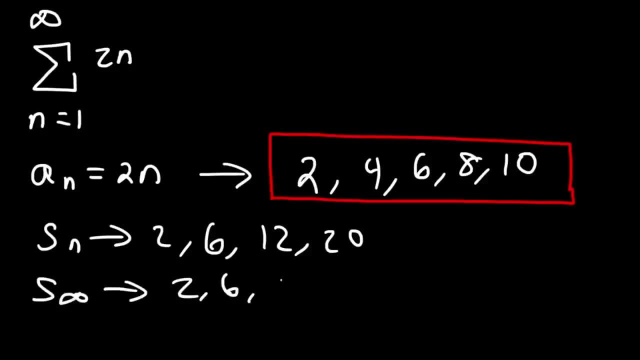 sequence goes into infinity. this will keep on going forever, And so this is termed an infinite series. So this is equal to s sub infinity. It's the sum of the first infinite terms. Now how can we tell if it's going to converge or if it's going to diverge? 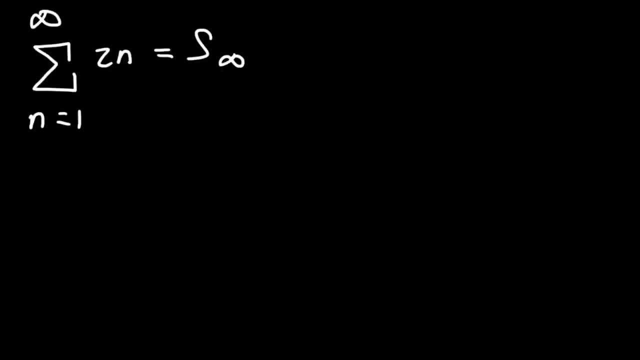 How can we find the answer? A more accurate way to describe this is to say that this is equal to the limit as n approaches infinity. So this is the sum of s sub n, which you could think of it as s sub infinity, but 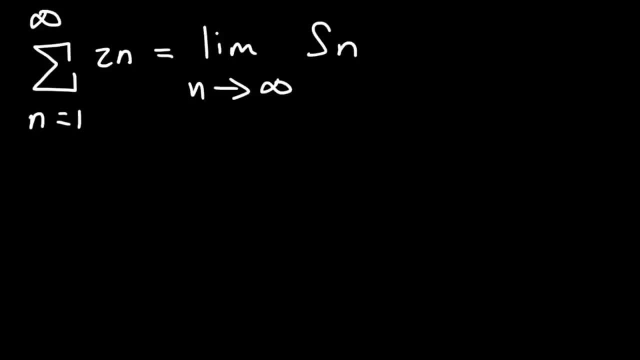 that might not be the most appropriate way to write it. So this means we're looking for the sum of an infinite number of terms. Now, in order to determine if the series converge, you need to know if the sum exists. Now let's go back to sequences. If you want to determine if the sequence is convergent, 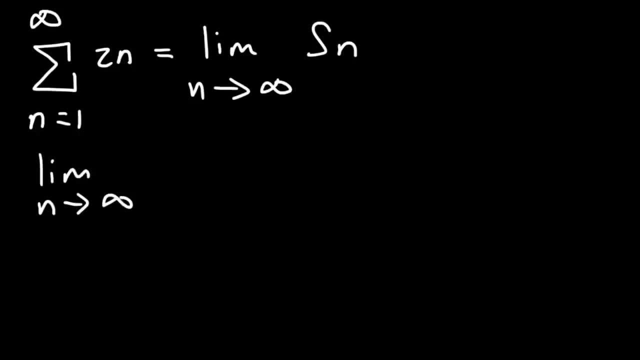 or not. what we need to do is take the limit, as n approaches infinity, of the sequence a sub n, and if it's equal to a constant, then we say that the sequence a sub n converges. Now, if the limit increases or decreases without bound, or if it 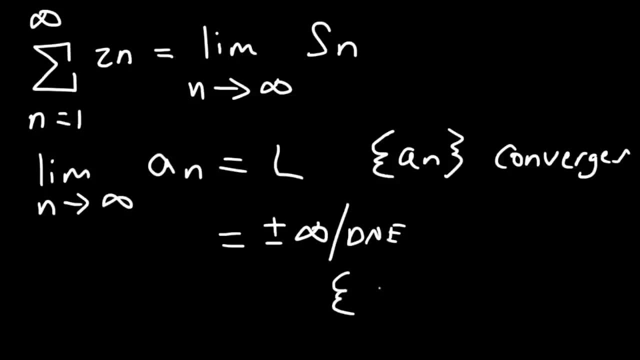 doesn't exist, then we say that the sequence a sub n it diverges. Now the same is true for a series, meaning the same concept is true. Now let's say if the infinite series or simply series, let's use a general. 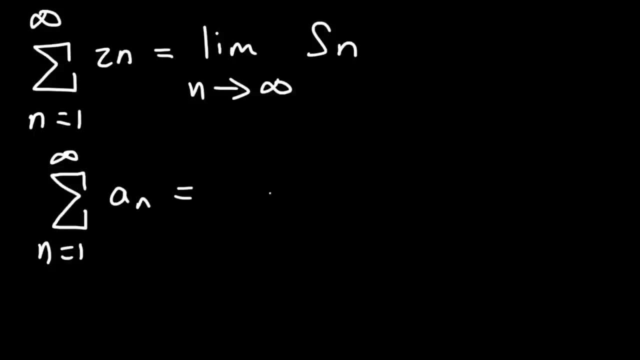 sequence. a sub n is equal to an actual number, which we'll call s. so that's the sum of the infinite series. then the series is convergent, It converges. But now let's say: if you can't determine the sum, Let's say: if the 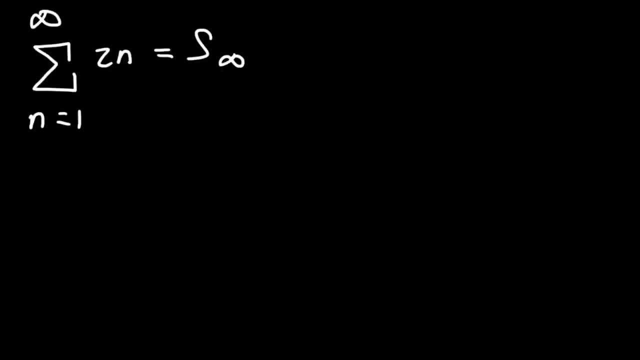 How can we find the answer? A more accurate way to describe this is to say that this is equal to the limit as n approaches infinity. So this is the sum of s sub n, which you could think of it as s sub infinity, but 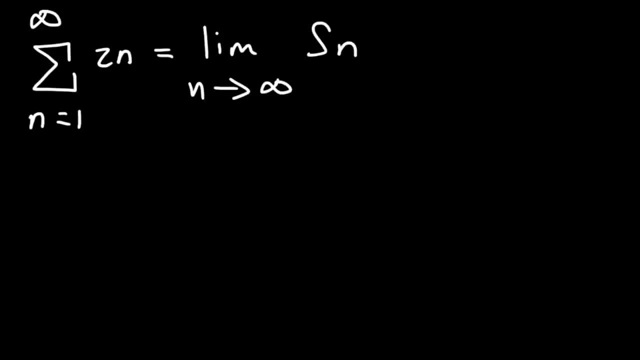 that might not be the most appropriate way to write it. So this means we're looking for the sum of an infinite number of terms. Now, in order to determine if the series converge, you need to know if the sum exists. Now let's go back to sequences. If you want to determine if the sequence is, 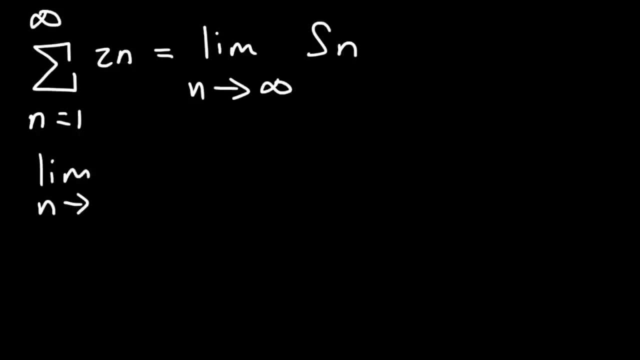 convergent or not. what we need to do is take the limit, as n approaches infinity, of the sequence a sub n, and if it's equal to a constant, then we say that the sequence a sub n converges. Now, if the limit increases or decreases without bound, or if it 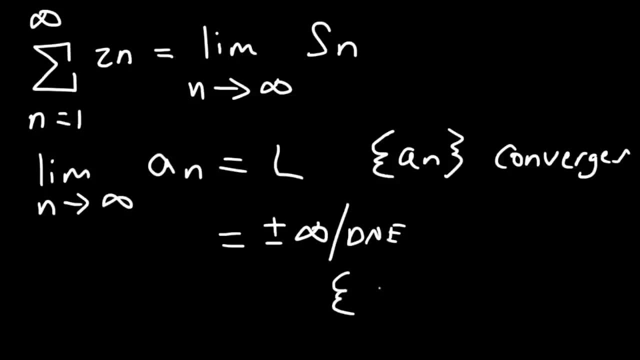 doesn't exist, then we say that the sequence, a sub n, it diverges. Now, the same is true for a series Meaning. the same concept is true. Now let's say if the infinite series, or simply series, let's use a general. 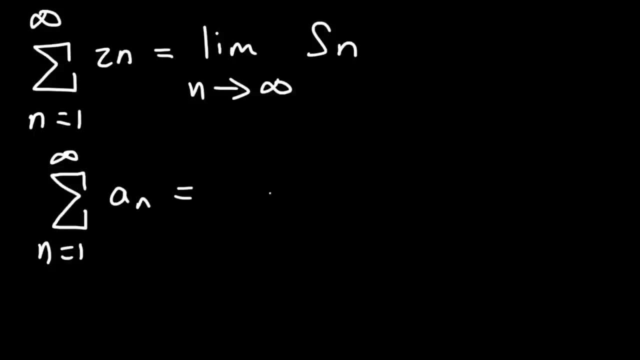 sequence. a sub n is equal to an actual number, which we'll call s. so that's the sum of the infinite series. then the series is convergent, It converges. But now let's say: if you can't determine the sum, Let's say: if the 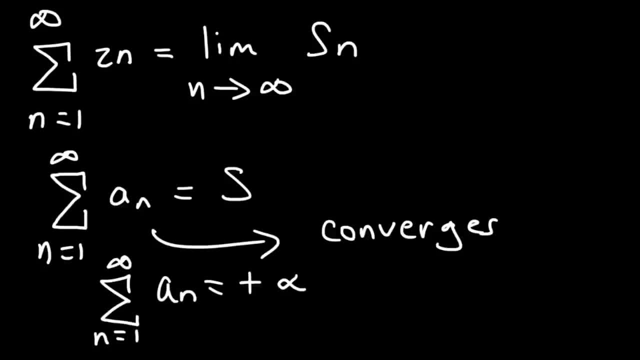 sum goes to infinity or something positive or negative infinity, then you can't really get a specific number there. so therefore the series diverges. So how can we determine the sum s? How can we know if it exists or not? Because if we can determine it, then we can determine if the series diverges. 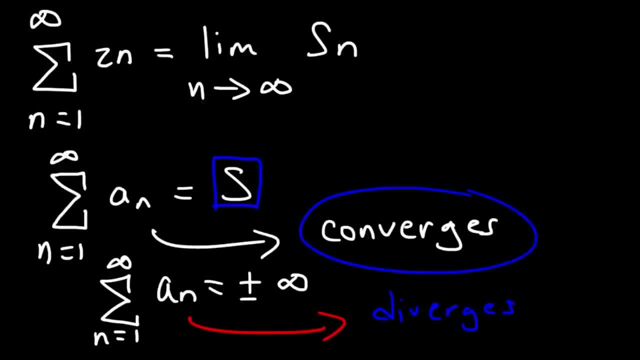 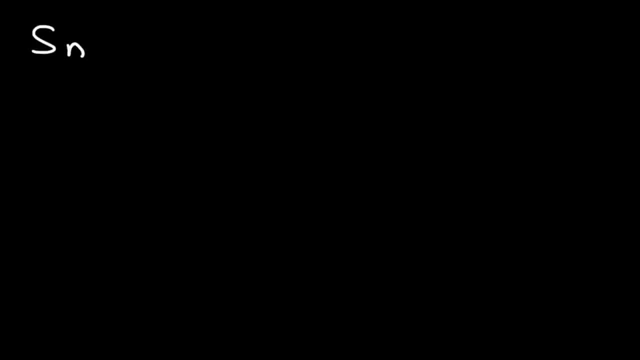 It's going to converge or diverge. So what you need to do is find a general equation for the partial sums s sub n, and it can vary depending on what situation you have. Once you have that, then you need to take the limit as n. 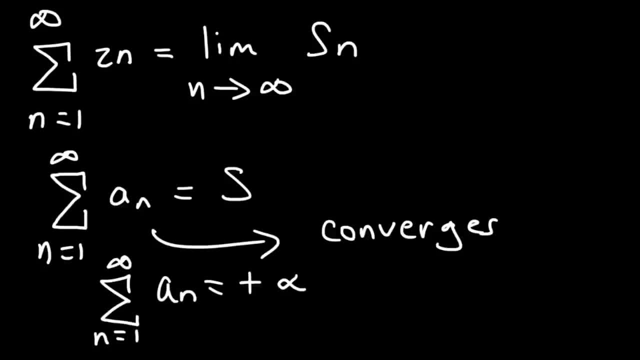 sum goes to infinity or something positive or negative infinity, then you can't really get a specific number there. so therefore the series diverges. So how can we determine the sum s? How can we know if it exists or not? Because if we can determine it, then we can determine if the series diverges. 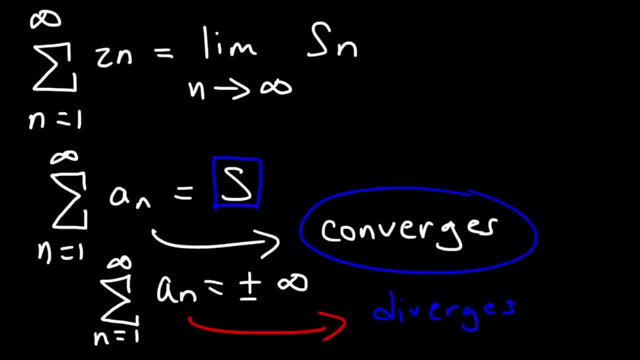 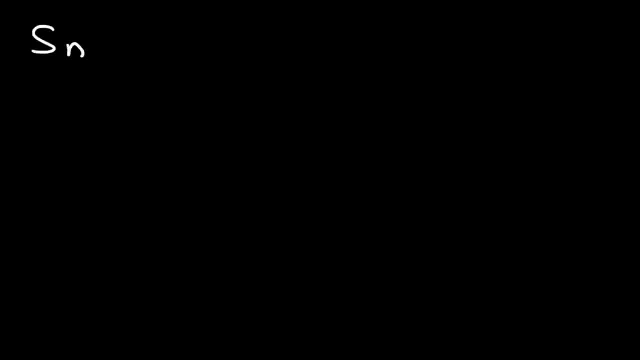 So what you need to do is find a general equation for the partial sums s sub n, and it can vary depending on what situation you have. Once you have that, then you need to take the limit. as n approaches infinity, for s sub n, This is equal to the infinite. 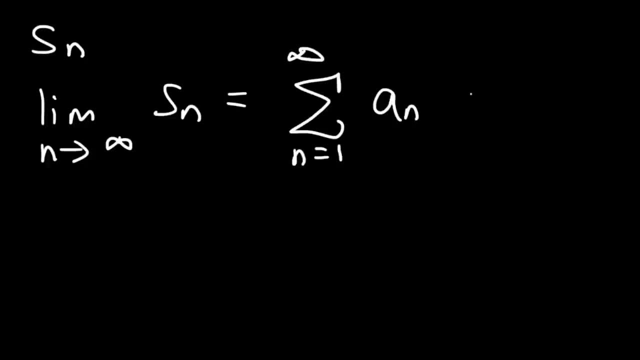 series, the sum of the infinite series. And so if you can actually get a number for this value and prove that it doesn't equal infinity or it doesn't exist, if you can get a finite value as n approaches infinity for some general 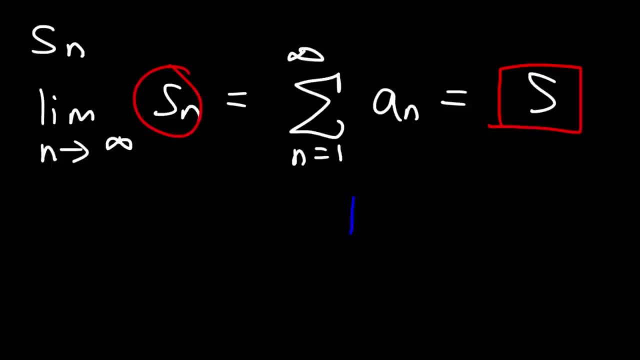 formula for s sub n, then you can show that the series converges. So let's start with this example: Determine if the infinite series converges or diverges This particular series. does it equal infinity or does it equal a number like 8?? If it's, 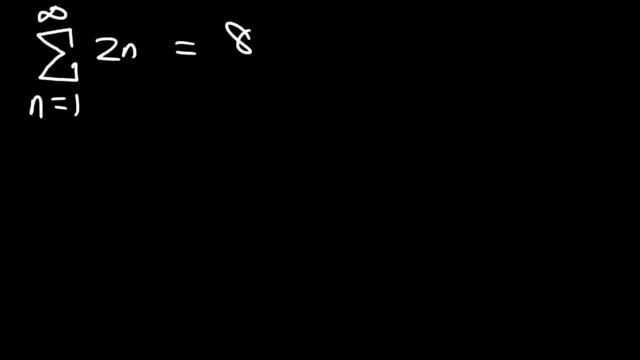 a specific number, it's going to converge. If it's infinity, it's going to diverge. Now let's think about what this means. So we know that a sub n is 2 n. If we list out the terms, the first term is going to be 2,. the second term is 4, the third term 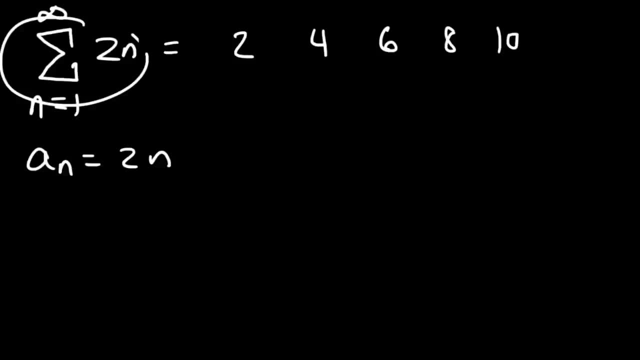 and then 8, and then 10. now we have a summation notation, so we're adding these terms and this will keep on increasing all the way to infinity. so just by looking at it, we know that the sum, the infinite sum, is infinity. just by looking. 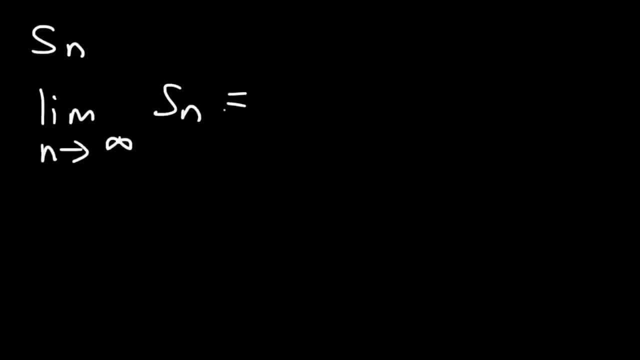 approaches infinity. for s sub n, This is equal to the infinite series, the sum of the infinite series. And so if you can actually get a number for this value and prove that it doesn't equal infinity or it doesn't exist, if you can get a finite value as n approaches infinity for some general 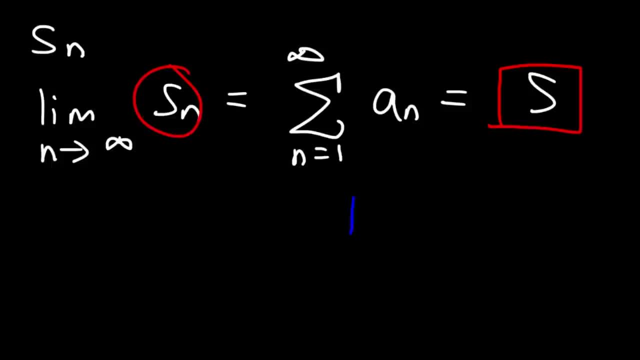 formula for s sub n, then you can show that the series converges. So let's start with this example: Determine if the infinite series converges or diverges. So this particular series, does it equal infinity or does it equal a number like 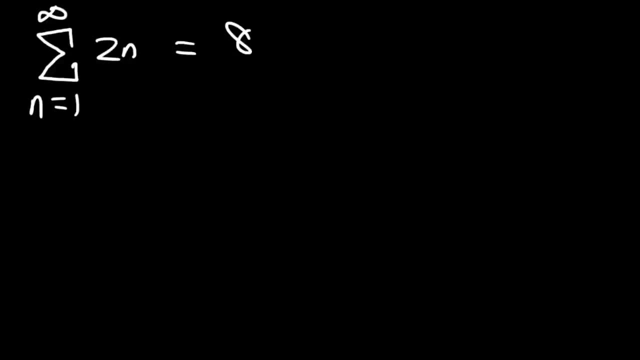 8?. If it equals a specific number, it's going to converge. If it equals infinity, it's going to diverge. Now let's think about what this means. So we know that a sub n is 2n, And so if we list out the terms, the first term is going to be 2,. 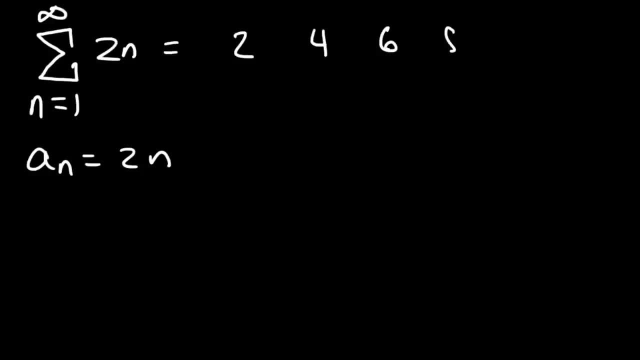 the second term is 4,, the third term is 6, and then 8, and then 10.. Now we have a summation notation, so we're adding these terms, And this will keep on increasing all the way to infinity. So just by 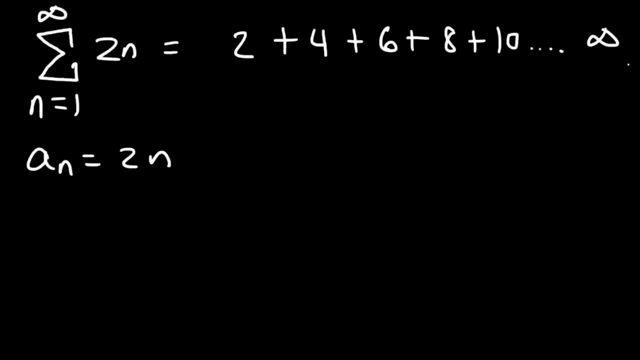 looking at it, we know that the sum, the infinite sum, is infinity, just by looking at it, intuitively. So that tells us that this series diverges. But let's see if we can confirm that answer another way. Now we need to determine a formula, s sub n for this particular series. Let's say: 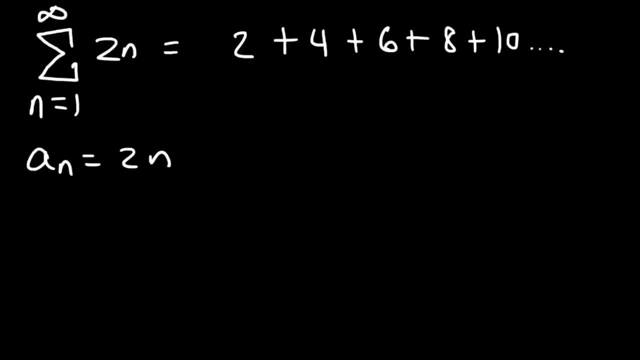 if we wish to determine the partial sum of the series up to some value n, How can we write a general formula for that? Well, you need to know what type of sequence you're dealing with. So here we're dealing with an arithmetic sequence. 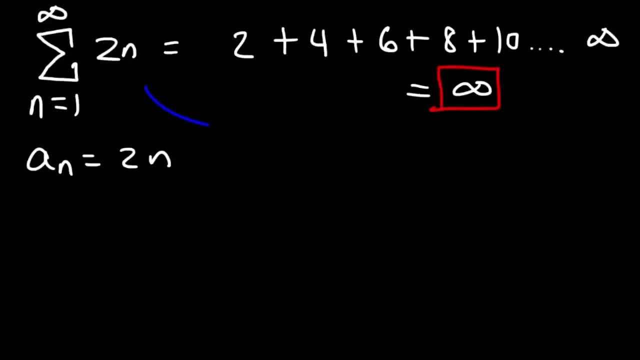 at it intuitively, so that tells us that this series diverges. but let's see if we can confirm that answer another way. now we need to determine a formula s sub n for this particular series. let's say, if we wish to determine the partial sum of the series up to some value n, how can 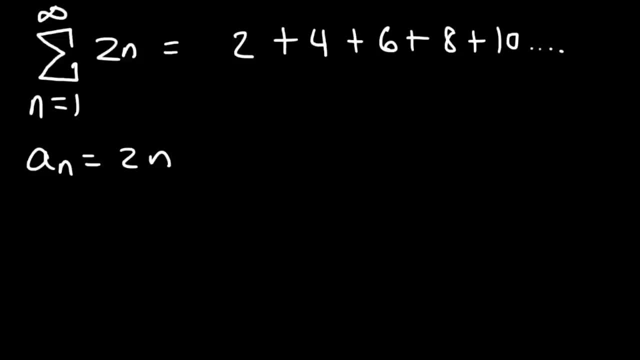 we write a general formula for that. well, you need to know what type of sequence you're dealing with. so here we go. we're dealing with an arithmetic sequence, and to find the partial sums of an arithmetic sequence you can use this formula: it's a sub 1 plus a sub n divided. 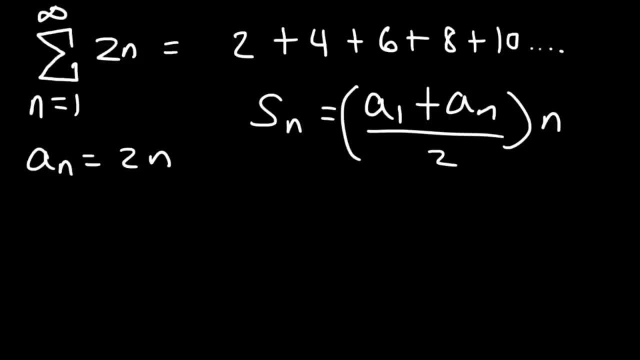 by 2 times the number of terms. now, a sub 1 is the first term, which is 2, a sub n. well, we have it here. it depends on what n is, so we're just going to write 2n and then there's an n out front. 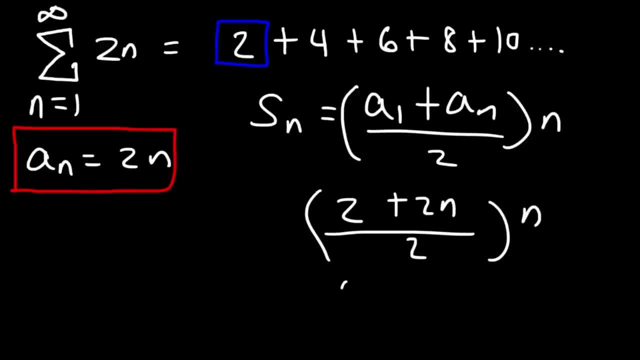 so 2 plus 2n divided by 2, that simply becomes 1 plus n or n plus 1. so our general formula for the partial sums its n times n plus 1. now let's take the limit as n approaches infinity for the partial sums s sub n, so that's the limit as n approaches infinity. and as s approaches end, so that's the limit as n approaches infinity. 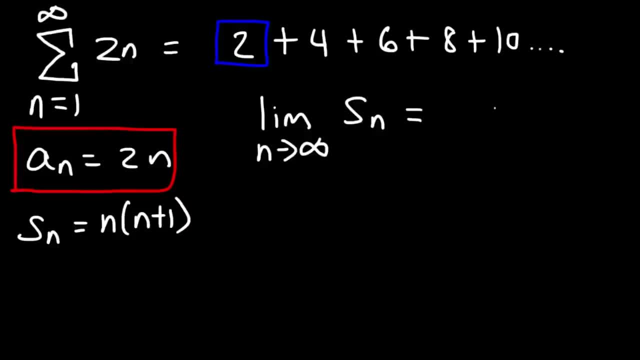 for the partial sums s sub n. So that's the limit as n approaches infinity of n, n plus 1.. So what does that equal? So if you have infinity times infinity plus 1, what will you get? A large number times a large number will give you an even larger number. So this is going to equal infinity. 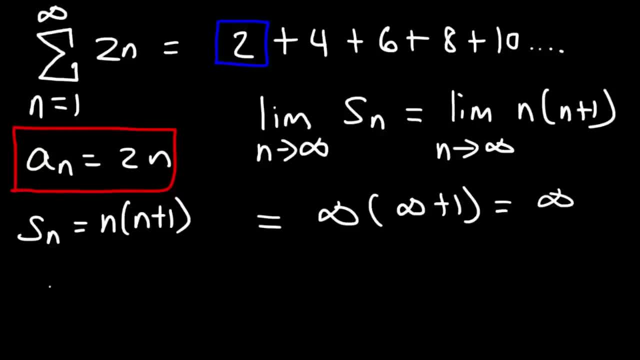 And so we could say that the infinite series that we have here. let's use the general formula, a sub n, that's equal to the limit as n approaches infinity. for the partial sums s sub n, And we found that it's equal to infinity, So it doesn't equal a finite number. 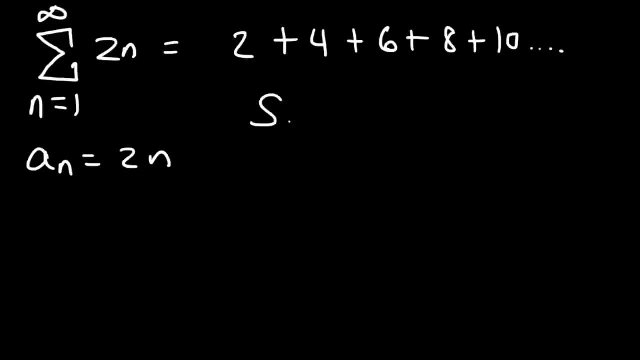 And to find the partial sums of an arithmetic sequence, you can use this formula: It's a sub 1 plus a sub n, divided by 2 times the number of terms. Now, a sub 1 is the first term, which is 2.. a sub n? well, we have it here. It depends on what n is. So we're just. 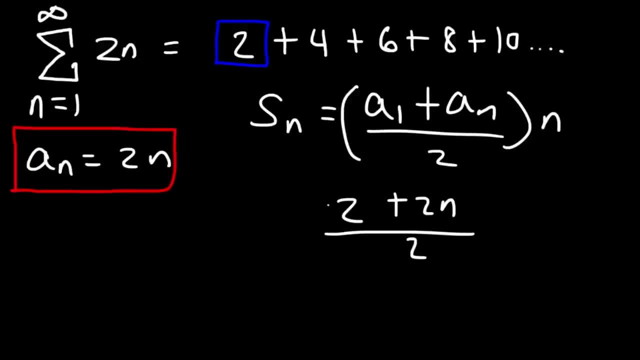 going to write 2n And then there's an n out front. So 2 plus 2n divided by 2, that simply becomes 1 plus n or n plus 1.. So our general formula for the partial sums is n times n plus 1.. 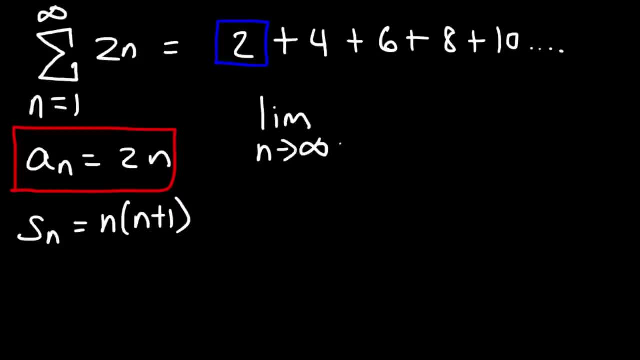 Now let's take the limit as n approaches infinity for the partial sums s sub n. So that's the limit as n approaches infinity of n n plus 1.. So what does that equal? So if you have infinity times infinity plus 1, what will you get? 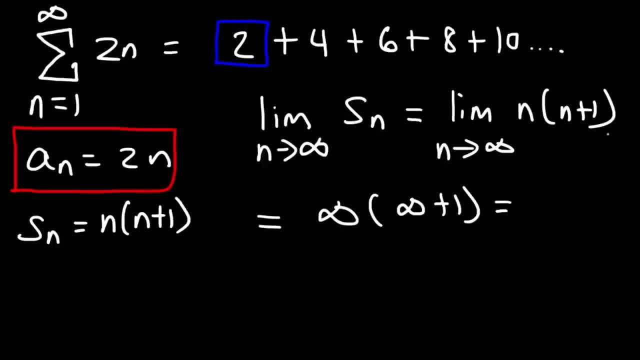 A large number times a large number will give you an even larger number. So this is going to equal infinity, And so we could say that the infinite series that we have here is going to equal infinity, And so we could say that the infinite series that we have here. 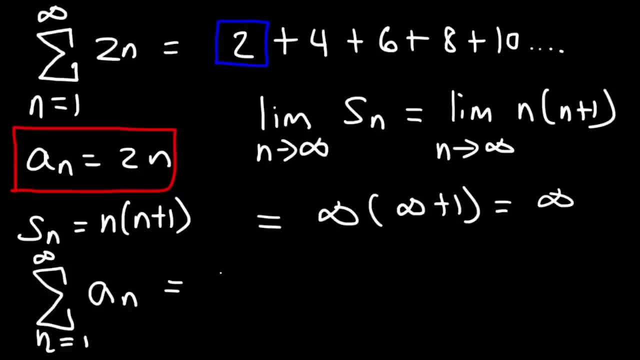 is going to equal infinity. Let's use the general formula a sub n. That's equal to the limit as n approaches infinity. for the partial sums s sub n, And we found that it's equal to infinity, So it doesn't equal a finite number. 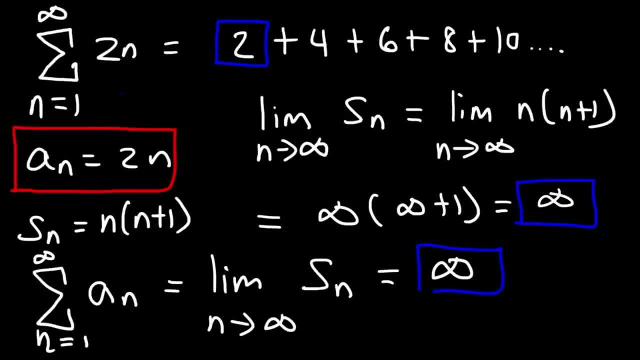 So, because it equals infinity, that tells us that the series, our original series, diverges, And so that's a more systematic way of determining if the series is going to converge or diverge. Find the sum. If the sum is infinity, it diverges. 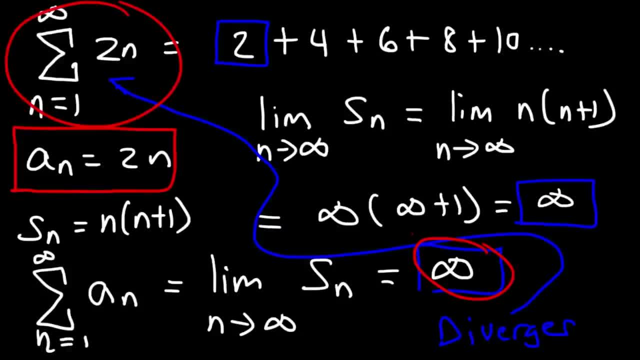 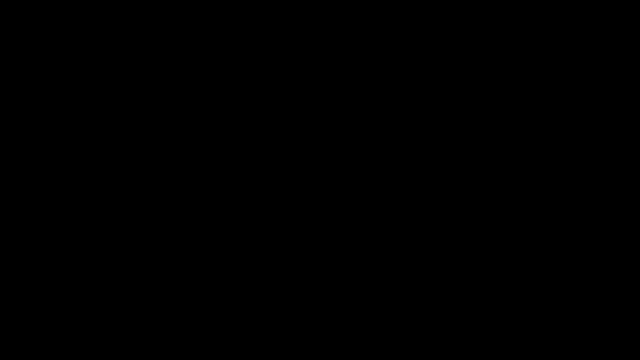 If it's equal to a finite number, it converges. Another test that is very useful, that can help you to quickly tell if a series diverges, is called the divergence test, And here's what it states. So let's say, if we have some sequence, a sub n. 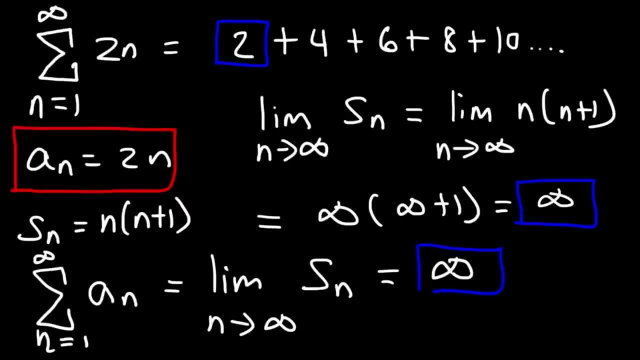 So because it equals infinity, that tells us that this series- original series- diverges, And so that's a more systematic way of determining if the series is going to converge or diverge. Find the sum: If the sum is infinity, it diverges If it's equal to. 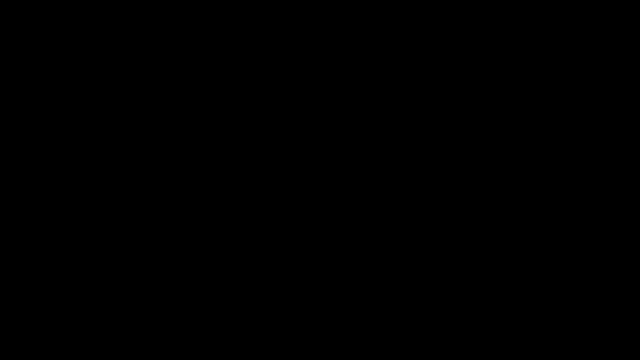 a finite number, it converges. Another test that is very useful, that can help you to quickly tell if a series diverges, is called the divergence test, And here's what it states. So let's say, if we have some sequence, a sub n. If the limit as n approaches infinity of the sequence, a sub n. 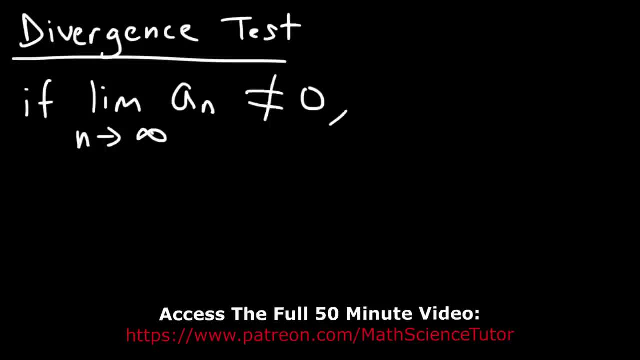 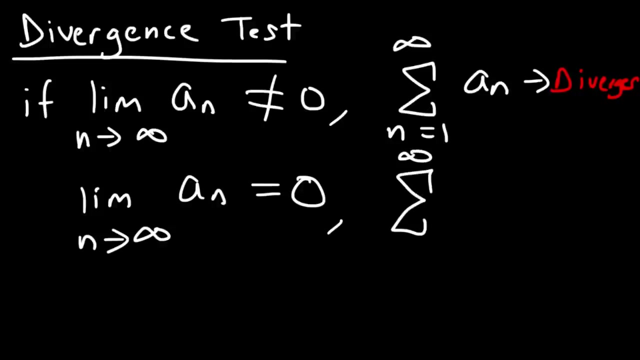 if it does not equal zero, then the series, the infinite series, diverges. So what about if it equals zero? So if the limit as n approaches infinity for the sequence, a sub n, let's say, if it's equal to zero, then the series, it may diverge or it may converge, We don't know. 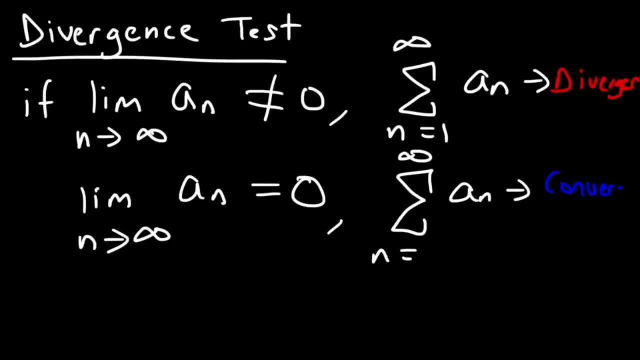 So we have to use other tests to figure it out. But the divergence test is a quick way to tell if it's going to diverge for sure or not. If it does equal zero, then you need to use another test to see if it's going to converge or diverge. 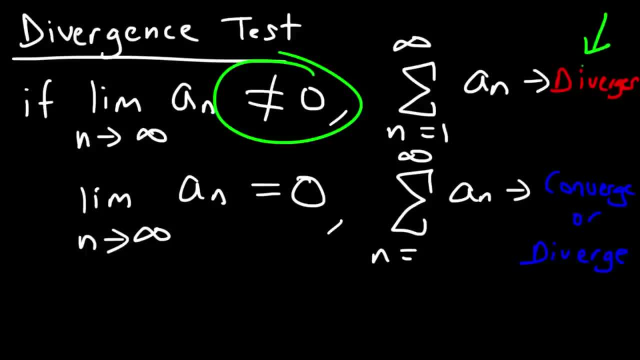 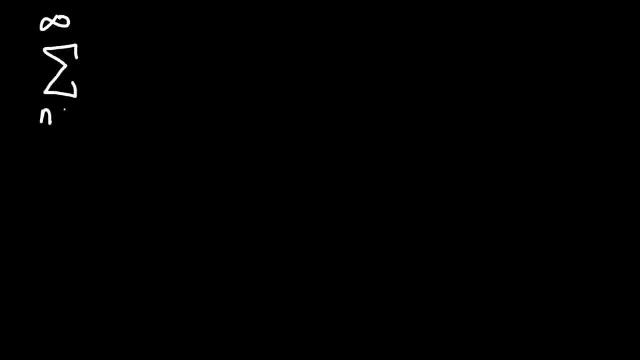 But if it doesn't equal zero, then automatically you know that it diverges. So let's go back to the first problem that we started with. Go ahead and use the divergence test to show that this series diverges. Now the first thing you need to do is determine a sub n. 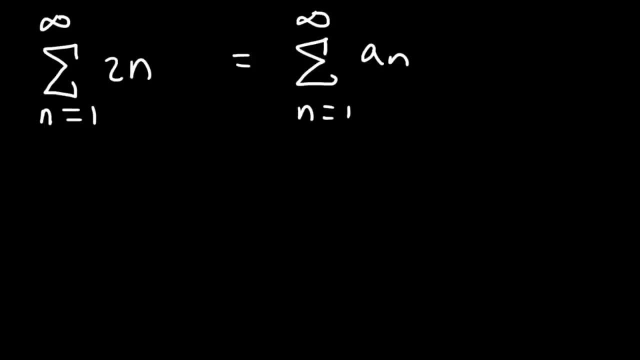 And so, as you know, a sub n in this problem is simply 2n. Next, take the limit as n approaches infinity of a sub n. So the limit as n approaches infinity for 2n. does that equal zero? It does not. 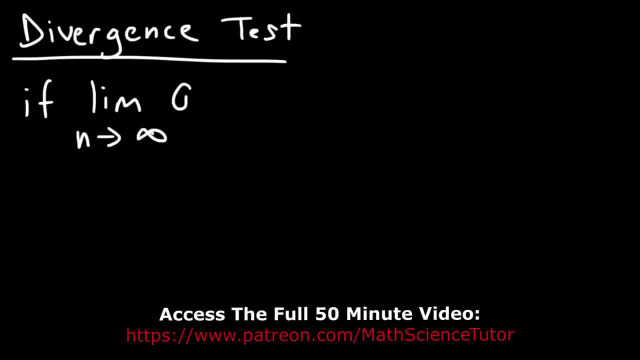 If the limit as n approaches infinity of the sequence, a sub n, if it does not equal zero, then the series, the infinite series, diverges. So what about if it equals zero? So if the limit as n approaches infinity for the sequence, a sub n, let's say, if it's a 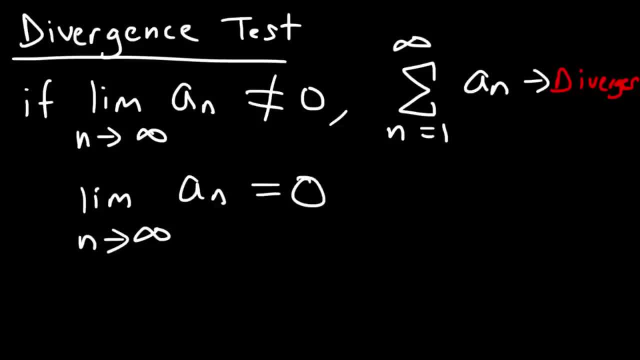 finite number equal to zero, then the series: it may diverge or it may converge, We don't know. So we have to use other tests to figure it out. But the divergence test is a quick way to tell if it's going to diverge for sure, or 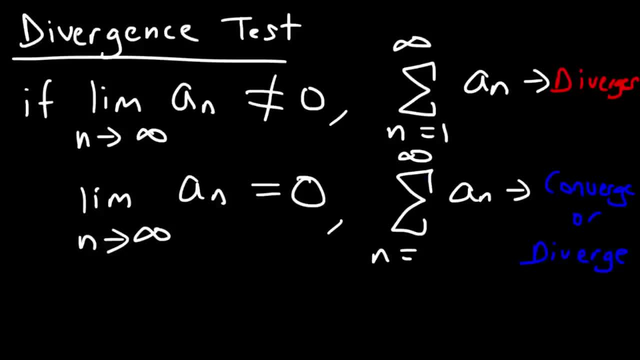 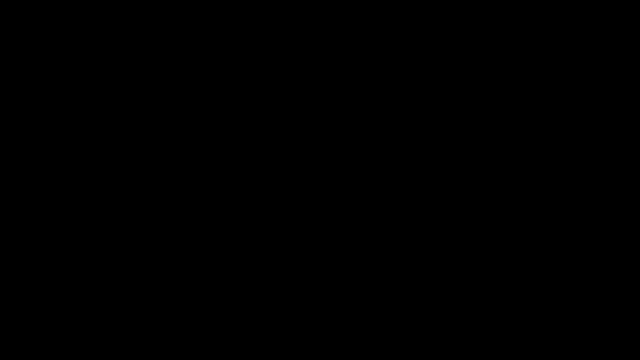 not. If it does equal zero, then you need to use another test to see if it's going to converge or diverge. But if it doesn't equal zero, then automatically you know that it diverges. So let's go back to the first problem that we started with. 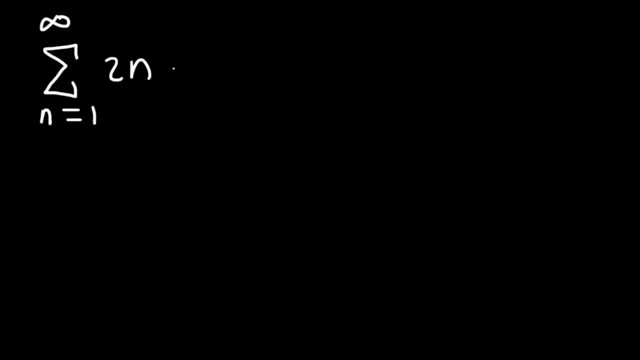 Go ahead and use the divergence test to show that this series is divergent. Now, the first thing you need to do is determine a sub n, And so, as you know, a sub n in this problem is simply 2n. Next take the limit. 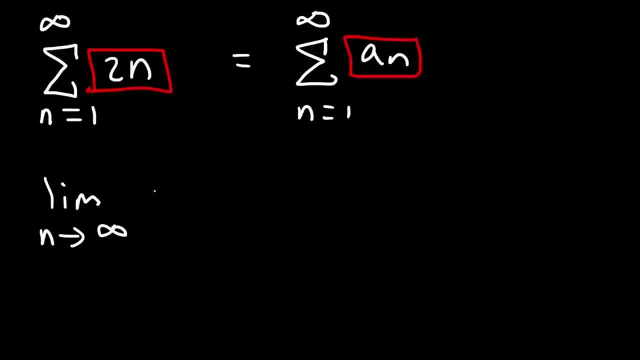 Take the limit as n approaches infinity of a sub n. So the limit as n approaches infinity for 2n. does that equal zero? It does not. 2 times infinity is equal to infinity. So since the limit as n approaches infinity for a sub n, because it does not equal zero, 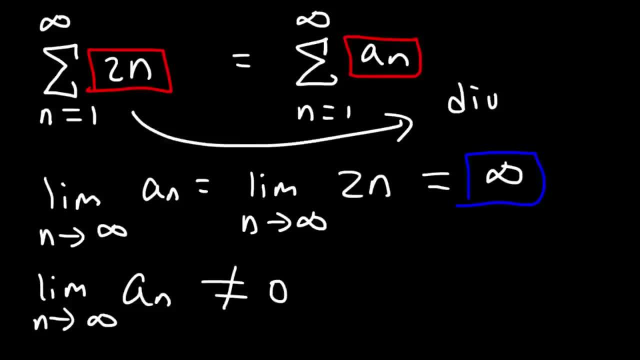 then we can say that the series diverges. Okay, So that's it, Thank you. And so, as you can see, it's a quick way to tell if it's going to diverge. If it did equal zero, then it may converge or diverge. 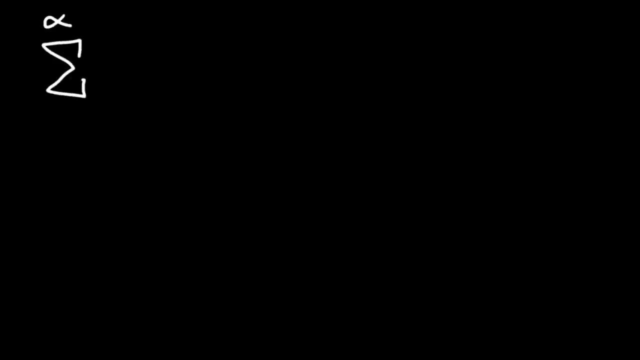 Here's an example that you could try Determine if the series converges or diverges. So the first thing I'm going to do is start with the divergence test. So we could see that a sub n is equal to 5n plus 3 over 7n. 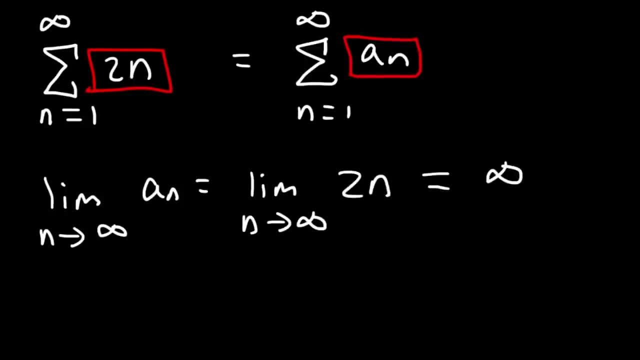 Two times infinity is equal to infinity. So the third question is: does it equal zero? So, since the limit as n approaches infinity for a sub n, because it does not equal 0, then we could say that the series diverges. And so, as you can see, it's a quick way to tell if it's going to diverge. 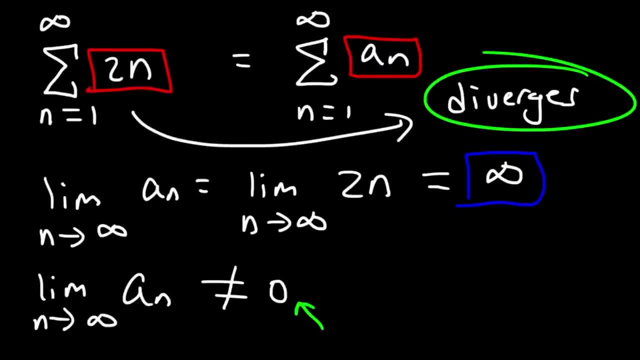 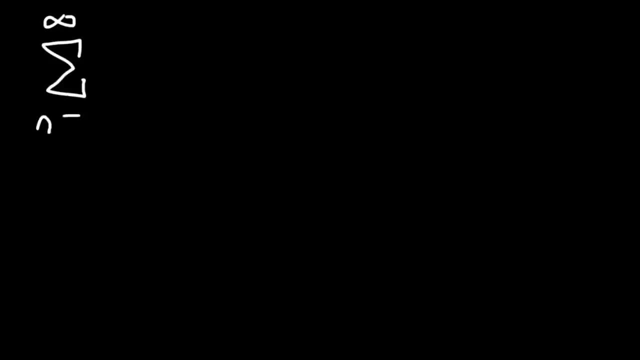 If it did equal 0, then it may converge or diverge. Here's an example that you could try Determine if the series converges or diverges. So the first thing I'm going to do is start with the divergence test. So we could see that a sub n is equal to 5n plus 3 over 7n minus 4.. 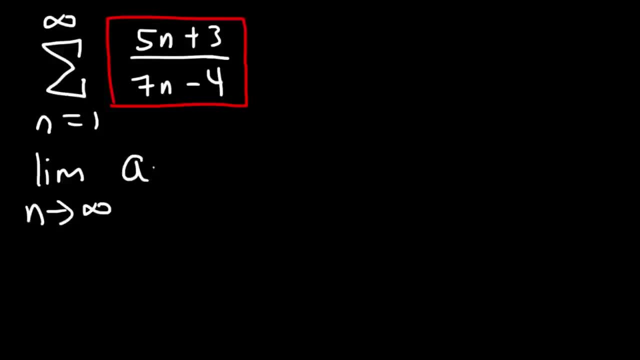 So what is the limit as n approaches infinity for a sub n? What answer will you get? So let's begin by multiplying the top and bottom by 1 over n. So we're going to have the limit as n approaches infinity, And this is going to be 5 plus 3 times 1 over n, divided by 7 minus 4 times 1 over n. 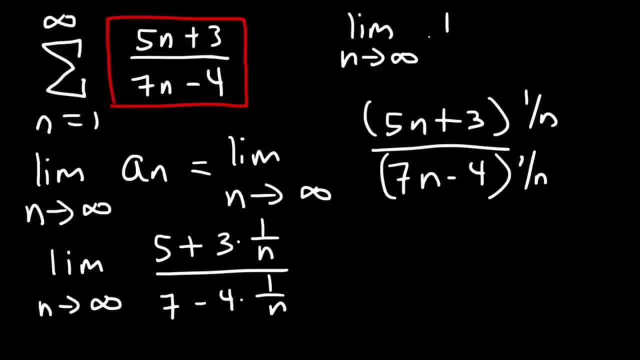 Now keep in mind the limit as n approaches infinity, for 1 over n will always be 0.. And 1 divided by a large number will equal a small number. So this becomes 5 plus 3 times 0 divided by 7 minus 4 times 0.. 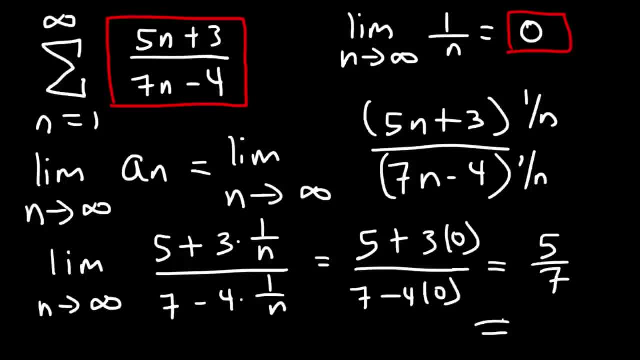 So this is equal to 5 over 7, which does not equal 0.. So therefore, because the limit as n approaches infinity, for a sub n, it does not equal 0, then we could say that the series it does not equal 0. 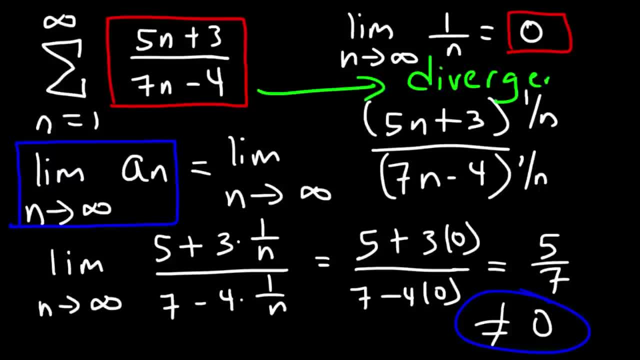 So the series diverges according to the divergence test. Now let's think about what this means. As n approaches infinity, the sequence a sub n converges to 5 over 7.. The sequence converges because the limit exists, But the series diverges because the sum at infinity. 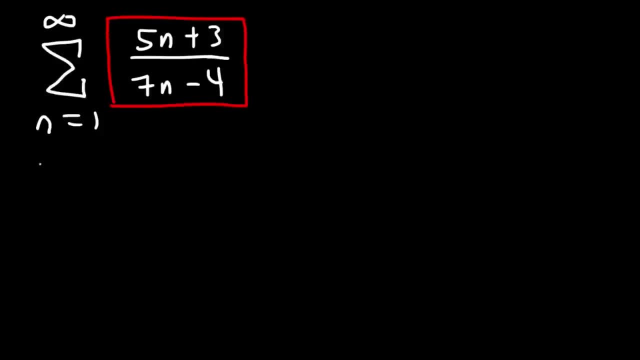 Okay, So what is the limit as n approaches infinity for a sub n? What answer will you get? So let's begin by multiplying the top and bottom by 1 over n. So we're going to have the limit as n approaches infinity. 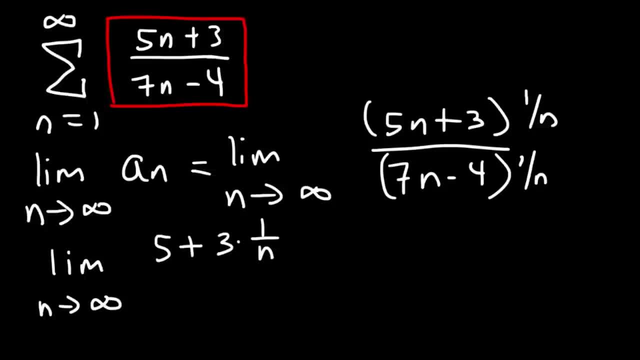 And this is going to be 5 plus 3 over 7.. Okay, 3 times 1 over n, divided by 7, minus 4 times 1 over n. Now keep in mind the limit as n approaches infinity, for 1 over n will always be zero. 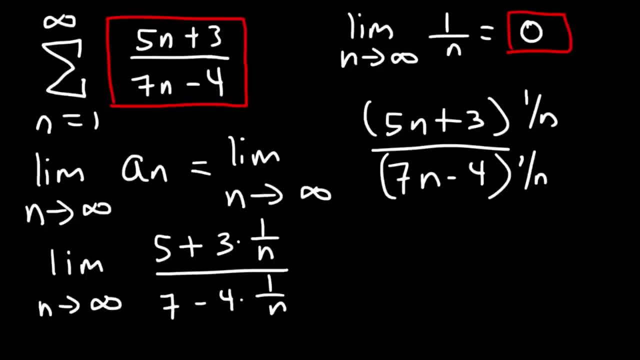 One divided by a large number will equal a small number. So this becomes 5 plus 3 times zero, divided by 7 minus 4 times zero, So this is equal to 5 over 7.. Which does not equal zero. So therefore, because the limit as n approaches infinity for a sub n, it does not equal zero. 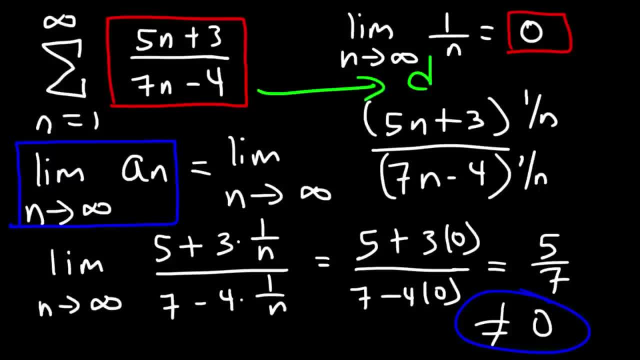 Then we could say that the series, it diverges according to the divergence test. Now let's think about what this means. As n approaches infinity, the sequence a sub n converges to 5 over 7.. The sequence converges because the limit exists. 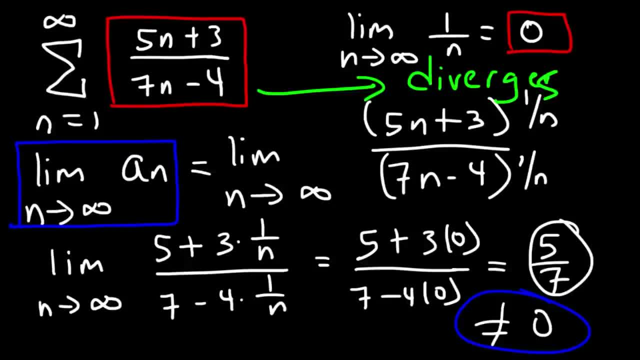 So what does that mean? Well, the series diverges because the sum at infinity doesn't equal a specific number. So in this problem- just keep in mind- the sequence is convergent, but the series is divergent. So if we think about what this really means, 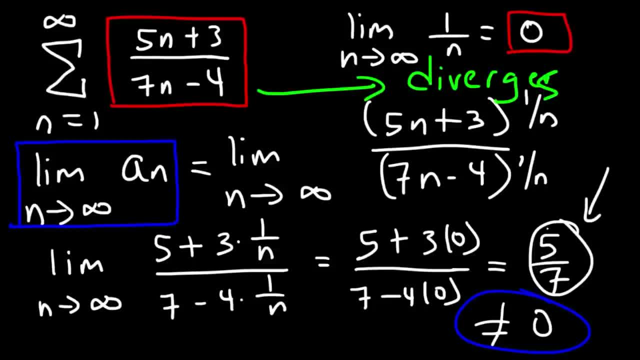 As we approach an infinite number of terms, we're going to keep adding 5 over 7 as n increases, And so if you keep adding 5 over 7 when n is very large, the sum will continue to change. It's going to get higher and higher and higher. 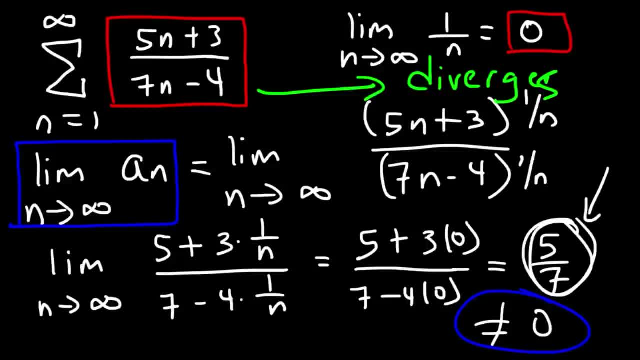 So it doesn't stay at a specific value. So any time the limit as n approaches infinity of a sub n, if it doesn't equal zero, the sum at infinity will keep going higher and higher and higher. The only way for the sum to stay at a finite value is to add zero. 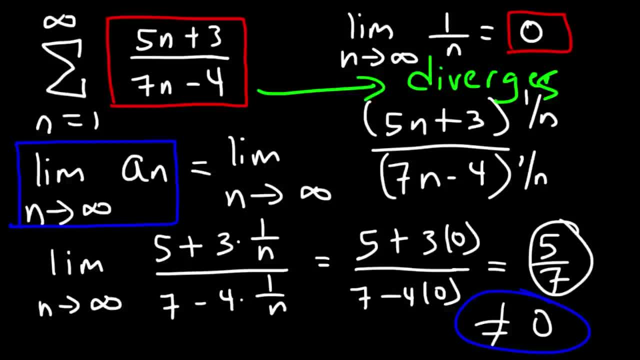 it doesn't equal a specific number. So in this problem, just keep in mind- the sequence is convergent but the series is divergent. So if we think about what this really means, as we approach an infinite number of terms, we're going to keep adding 5 over 7 as n increases. 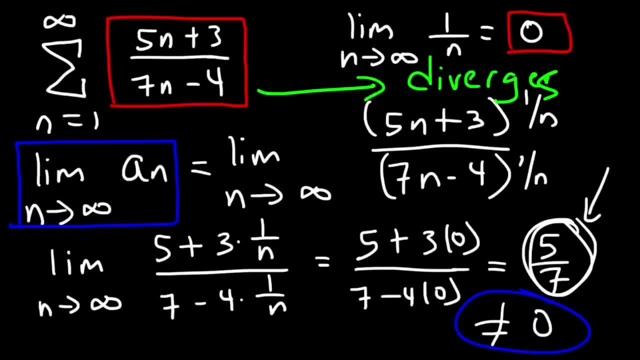 And so if you keep adding 5 over 7 when n is very large, the sum will continue to change. It's going to get higher and higher and higher, So it doesn't stay at a specific value. So any time the limit as n approaches infinity of a of n, 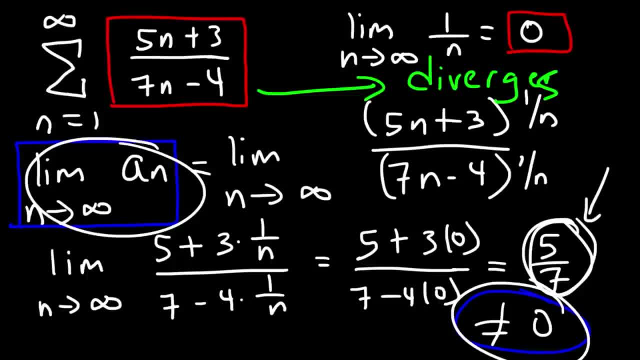 if it doesn't equal 0, the sum at infinity will keep going higher and higher and higher. The only way for the sum to stay at a finite value is to add 0. Let's say the finite value is 100.. Let me use an example. 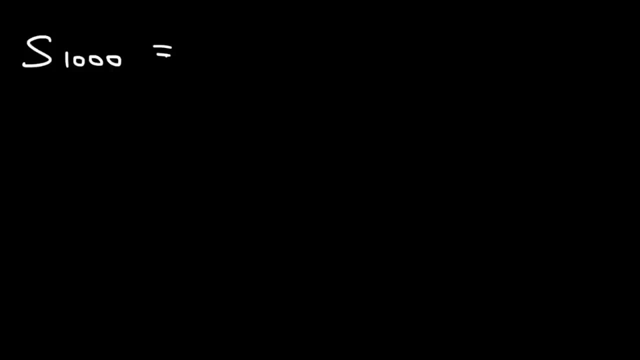 So let's say s of 1000 is 200. And let's say the limit as n approaches infinity for this sequence is 5.. So let's say, at a of 1000, it's also approximately 5.. So s of 1001 will be 205 approximately. 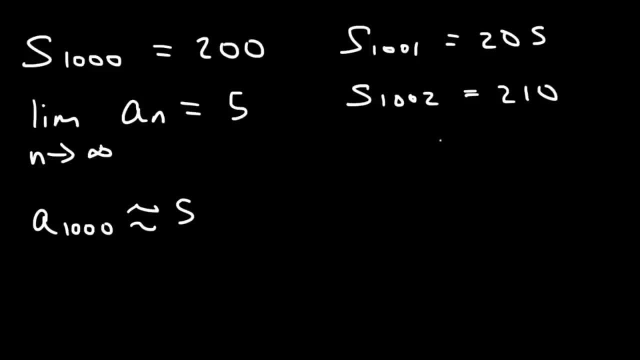 S 1002 would be 210.. And so the sum will continue to go up as n increases. So therefore, this will never stop at a specific value. Now let's say: let me get rid of this stuff. Let's say, if the limit as n approaches infinity for a sub n did equal to 0. 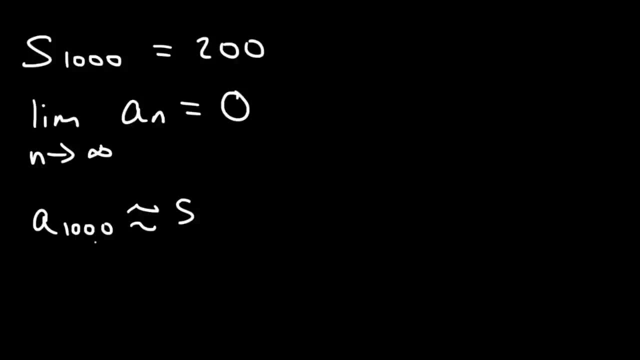 Then let's say a of 1000 is approximately 0. It might be like .001,, but let's say it's close to 0. Then s of 1001 is going to approximately be 200.. s of 1002 will still be 200.. 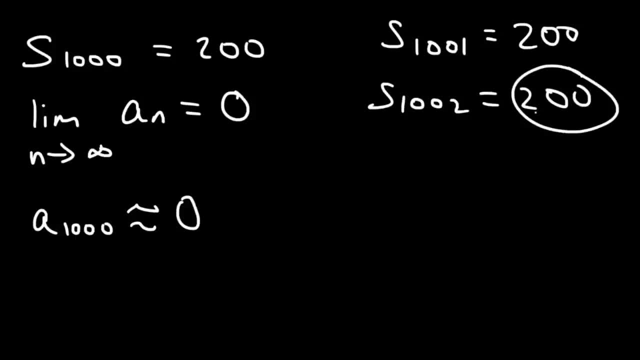 Because if you keep adding a small number to this that keeps getting closer and closer to 0,, it's going to stay at approximately 200.. In that case, the sum converges, And so that's why, in order for the series to converge, 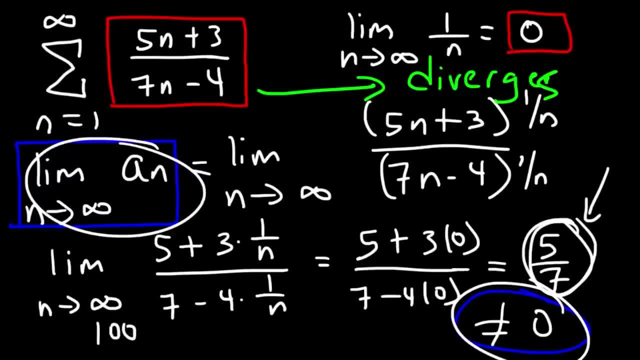 Let's say the finite value is 100.. Let me use an example. So let's say S of 1000 is 200.. And let's say S of 1000 is 100.. Let's say S of 1000 is 200. 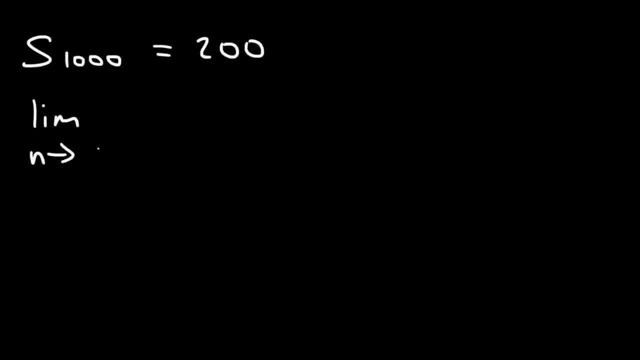 Let's say S of 1000 is 200.. Let's say: the limit as n approaches infinity for this sequence is 5.. So let's say at A of 1000, it's also approximately 5.. So S of 1001 will be 205 approximately. 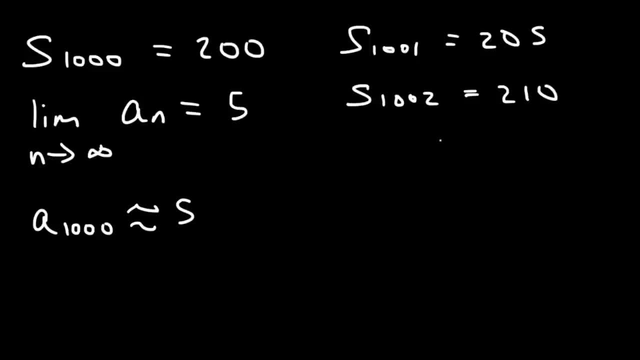 S 1002 would be 210. And so the sum will continue to go up as n increases. So therefore, this will never stop at a specific value. Now let's say: let me get rid of this stuff. Let's say, if the limit as n approaches infinity, for a sub n did equal to zero. 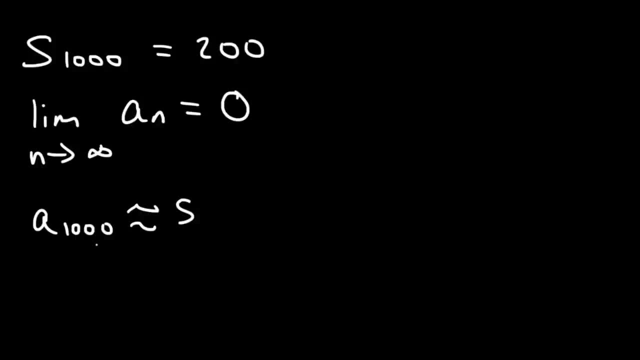 Then let's say A of 1000 is approximately zero. It might be like .001,, but let's say it's close to zero. Then S of 1000 is approximately 0. It might be like .001,, but let's say it's close to zero. 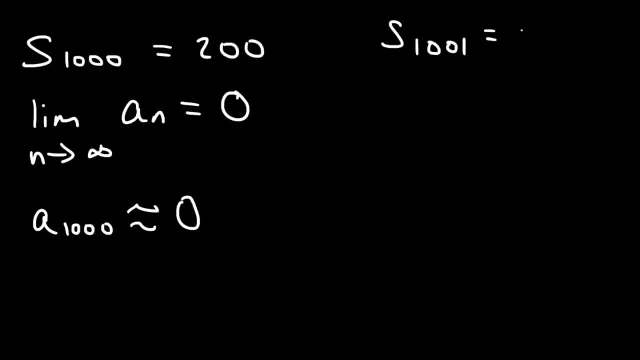 Then S of 1000 is approximately 0.. Then S of 1000 is approximately 0.. S of 1001 is going to approximately be 200.. And S of 1002 will still be 200.. And S of 1002 will still be 200.. 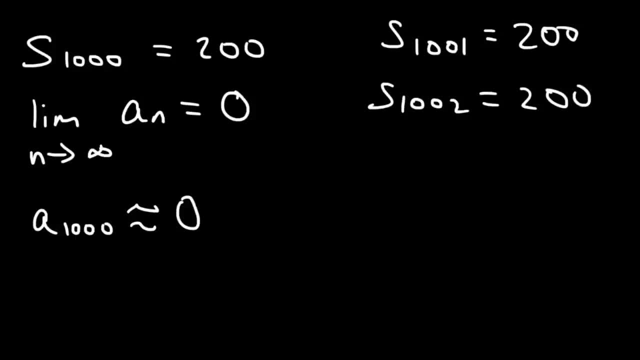 And S of 1002 will still be 200, because if you keep adding a small number to this that keeps getting closer and closer to zero, it's going to stay at approximately 200.. In that case, the sum converges, And so that's why, in order for the series to converge, the limit as n approaches infinity. 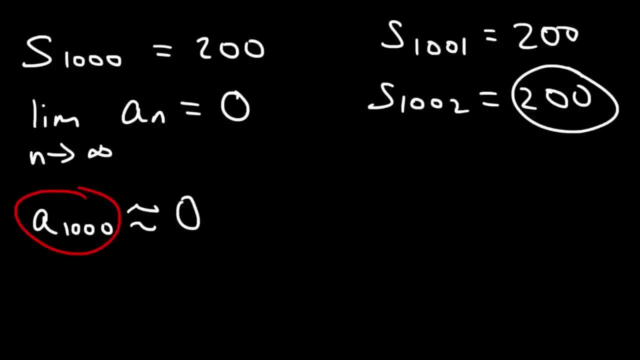 for A sub n. So when you have a very high term, it has to be a close to zero, Otherwise the sum will continue to increase. So if you want the sum to stay at a finite value, you have to keep adding 0 to it. 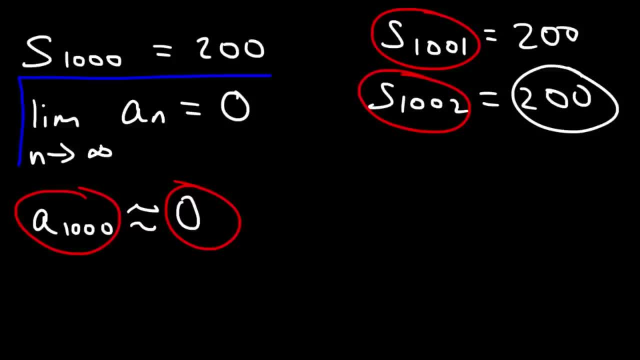 So in order for the series to converge, this must be equal to 0. But if it doesn't equal 0, then it has to diverge. If it does equal 0,, keep in mind it may converge or it may diverge. 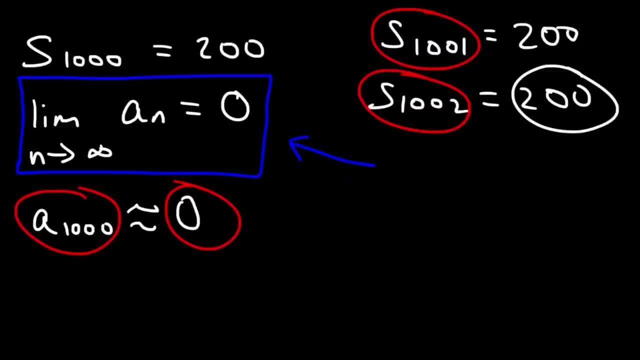 The series doesn't have to converge, but it may converge or the series may diverge.